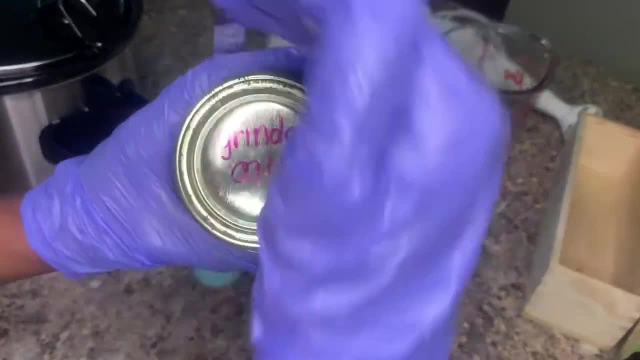 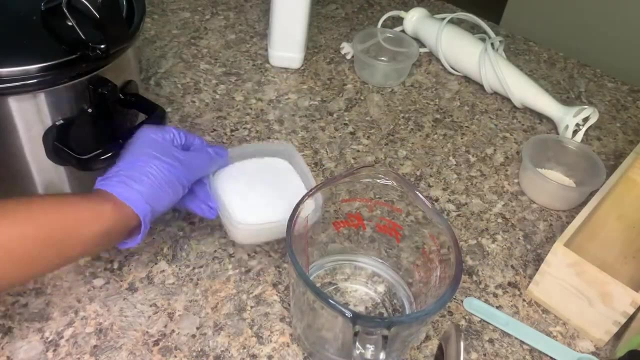 And 4.42 ounces of sodium hydroxide, aka lye. Now I'm just preparing everything. for the end, This is going to be one tablespoon of colloidal oatmeal, And I'm going to set that to the side and start preparing my live water. 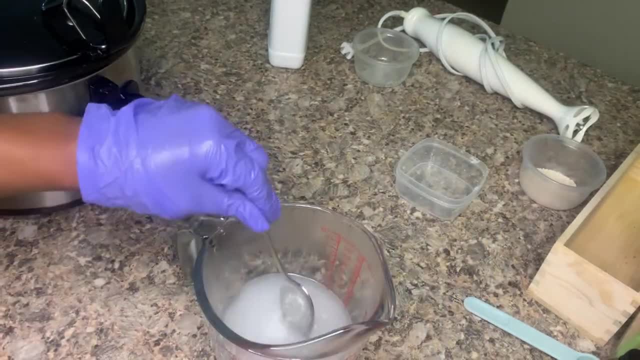 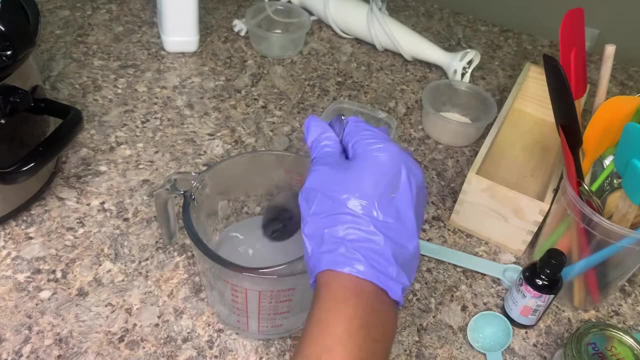 You want to make sure you always pour the lye into the water, Never the water into the lye. Think about it like the lye goes into the water And you want to just stir it and let it cool down a bit. Now I like to use sodium lactate to help my bar. 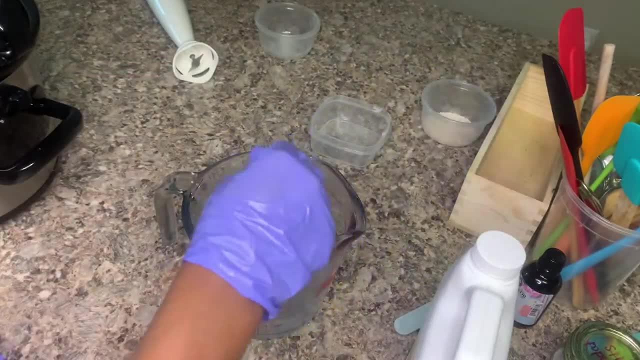 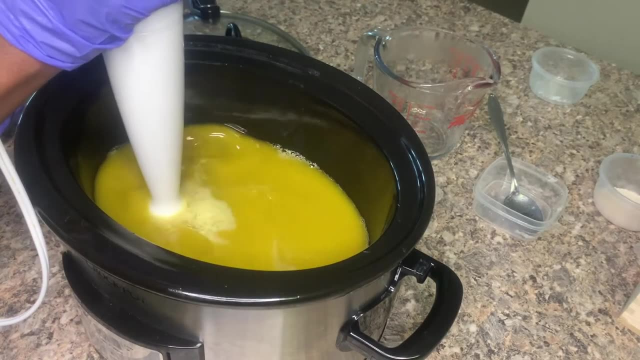 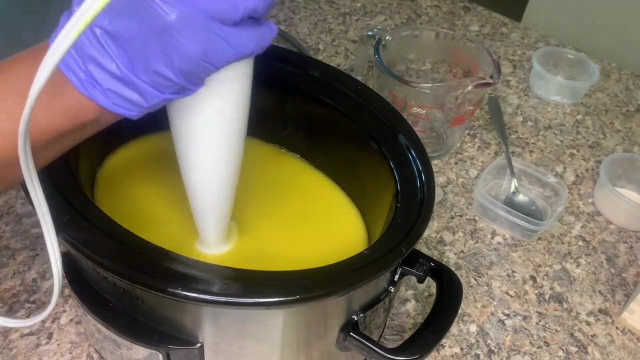 To help my bars last longer. For this recipe, you can use one teaspoon of sodium lactate. Now you're going to mix your lye water with your melted oils And you're going to bring your soap to a trace. If you haven't already, go check out my last video, which is a how to know when your soap has reached trace with the hot process soap method. 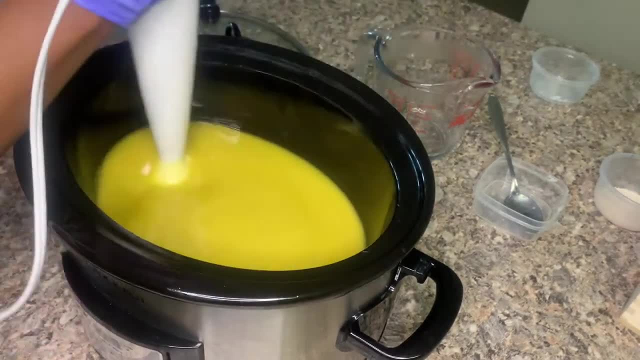 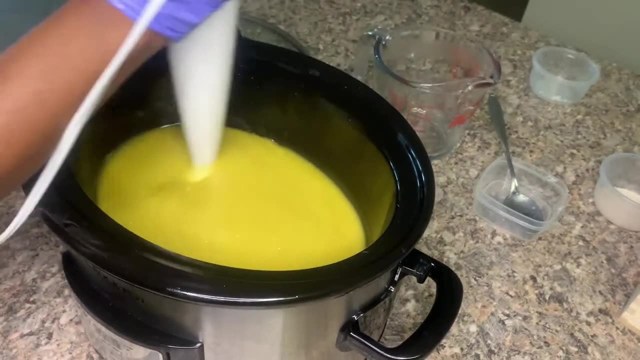 Now what I do is I always make sure it's come to trace because if you don't, your soap will burn people's skin because it will be lye heavy. So bringing your soap to trace is important. It's very, very, very, very important. 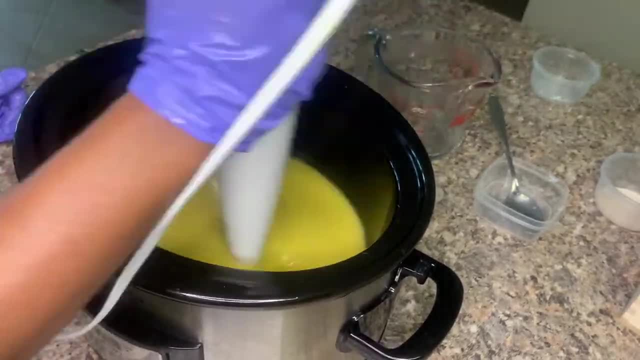 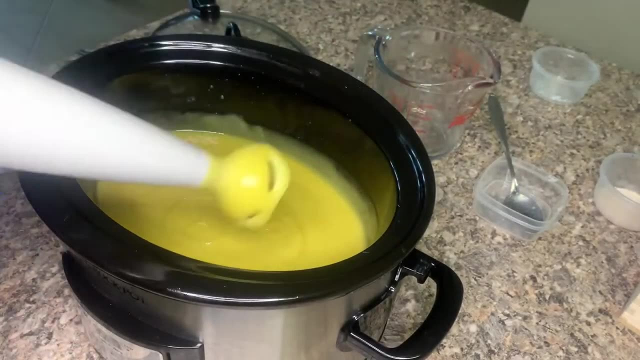 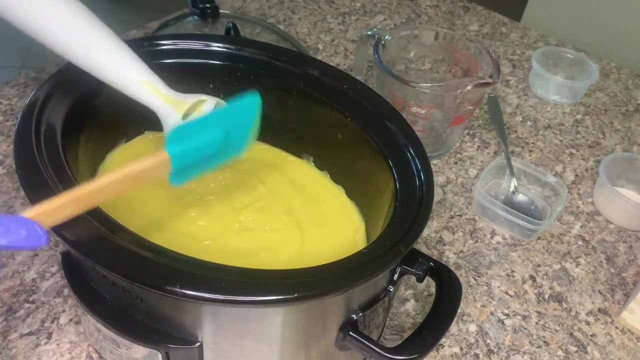 Don't sleep on it. Now that my soap has come to trace, I'm just going to get all of that down there, Scrape it off the stick blender, Get all of my soap. Every piece of soap mixture counts. No soap left behind. 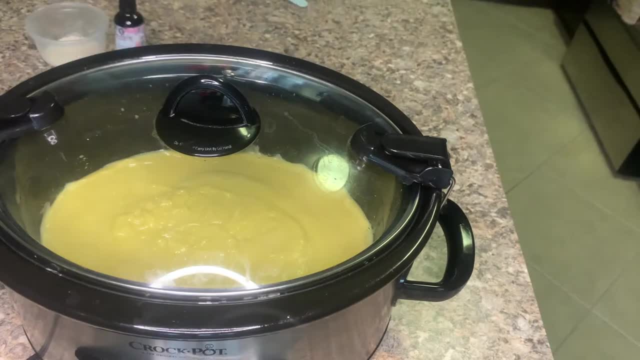 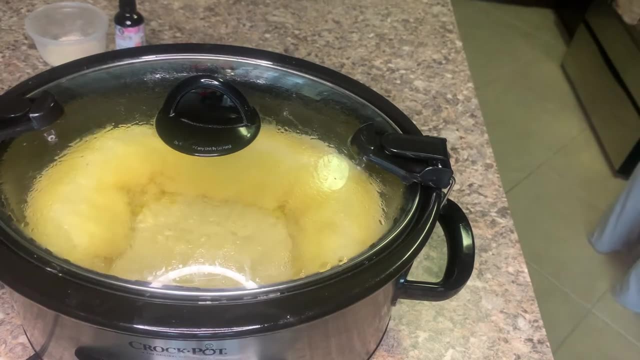 Put the top on And let your soap cook down. I have this super cool video right now of it sped up where you can see the soap cooking. Sometimes when you're cooking soap, the soap will start to volcano out of the crock pot and you might have to open it really quick and stir it down to not let it overflow. 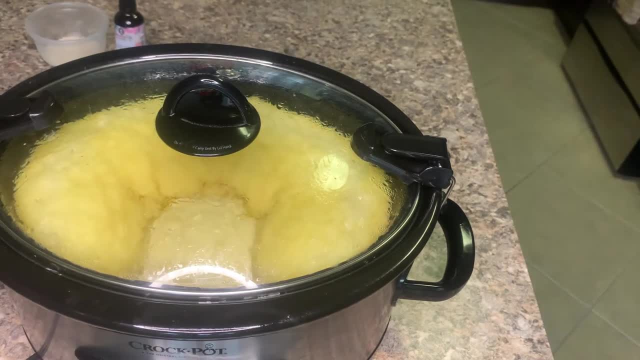 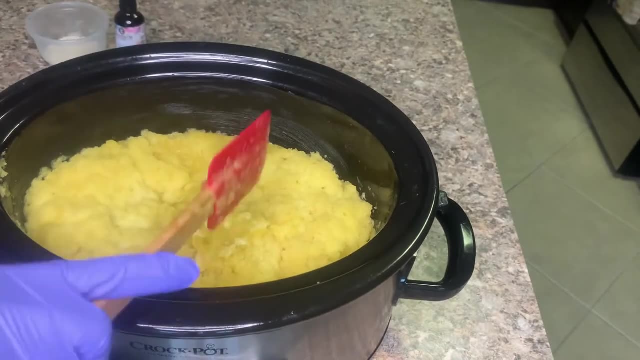 So, as you can see on the side, I'm getting my next set of gloves to get ready to stir that down. And one thing I've learned in hot process soap making is you want to open your crock pot as little as possible. You don't want any of the moisture to evaporate out of the soap. 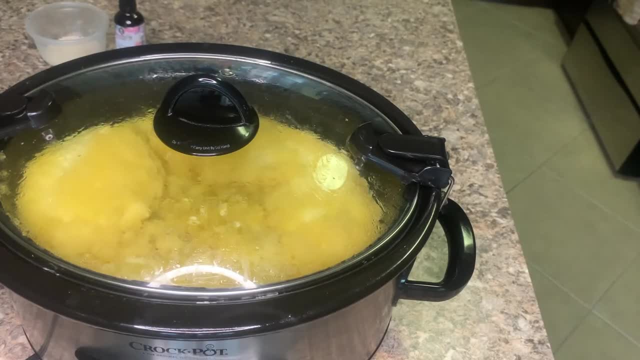 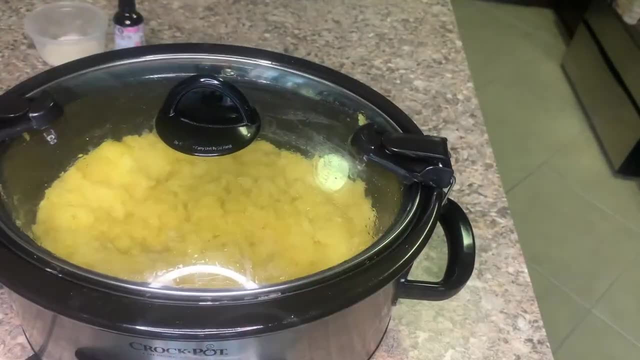 That is a really, really, really big secret, But the only time I ever stir in my soap is when I have to stir it down because it is volcanoing out. So yeah, you're going to let your soap cook down and I'll be back when it's time to mold the soap. 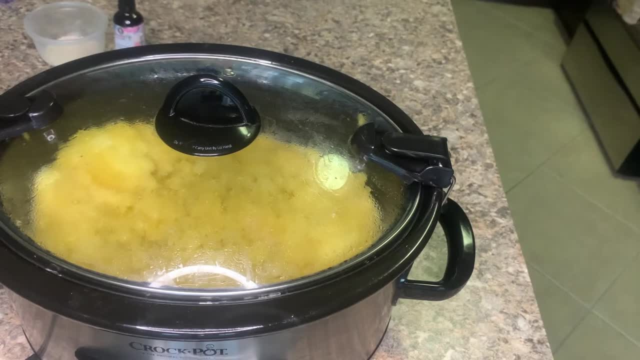 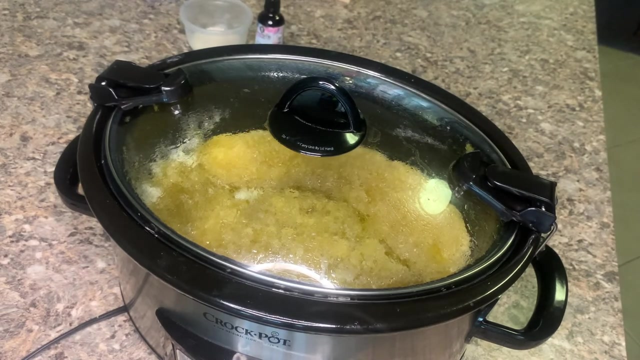 Make sure your consecrations are correct. Keep me posted. Have a great week today. I really hope that you enjoyed my video. Thank you for watching. Keep making me happy. I love you. so, as you can see, the soap is pretty much finished. I've tested it to see if. 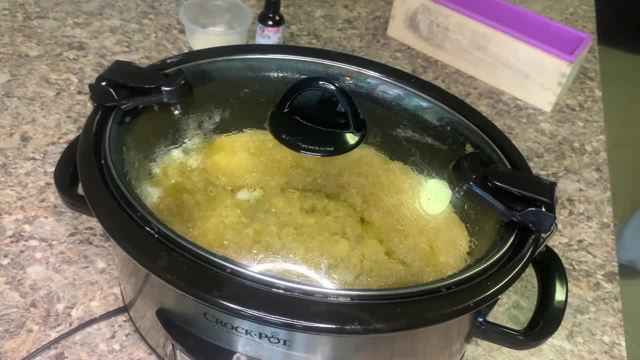 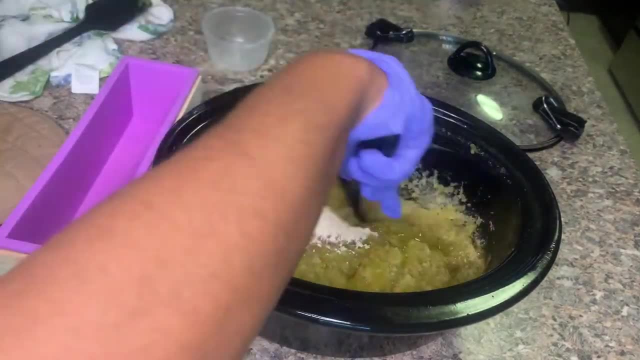 it was done and I am about to take it out and mold it. so I'm gonna add my colloidal oatmeal that I prepped earlier and I'm gonna stir it fast. you know times of the essence when you're making hot processed soap. you don't want the 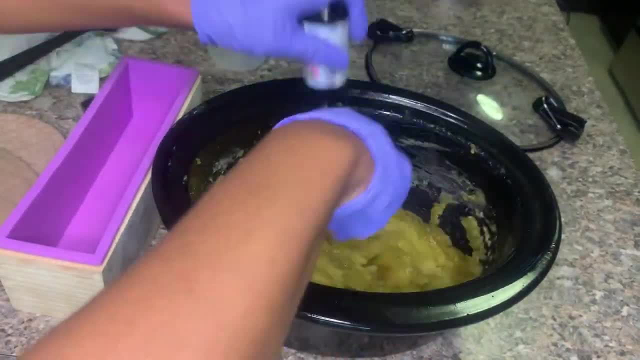 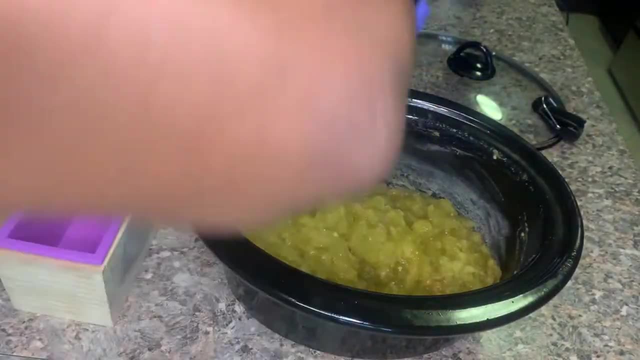 soap to get too cool. so what you have to do, that's the fragrance oil for this, for this specific soap. so what you have to do is you have to move as fast as you can. that's why I like to prep everything beforehand, so I'm not looking and the 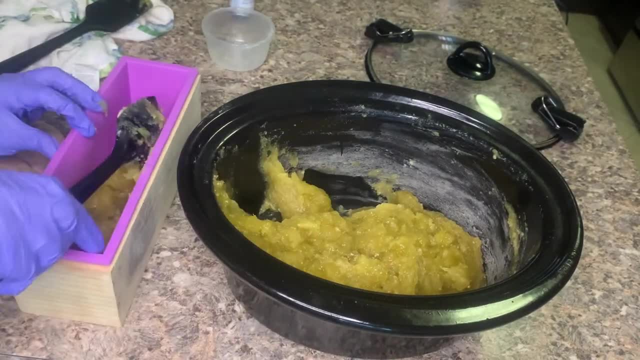 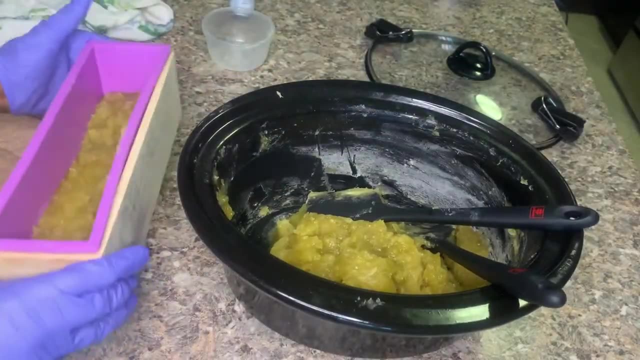 soap isn't cooling down, so I'm just stirring it, getting it in there, and I'm going to put it in the mold. when you're molding soap, you want to put stuff in and then shake the mold right there onto onto the countertop so that you can. 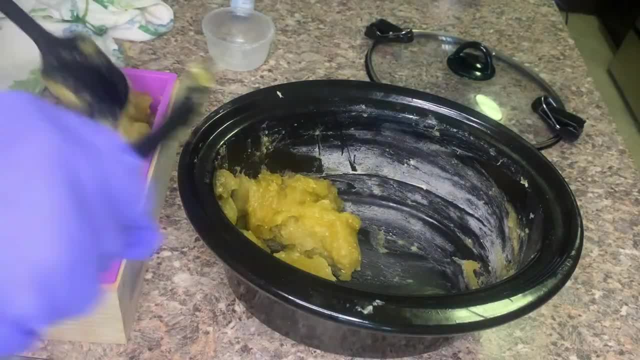 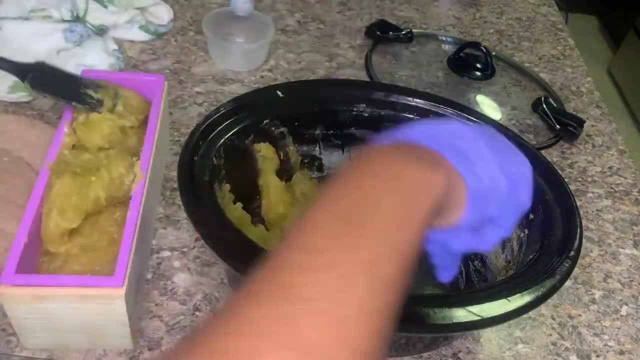 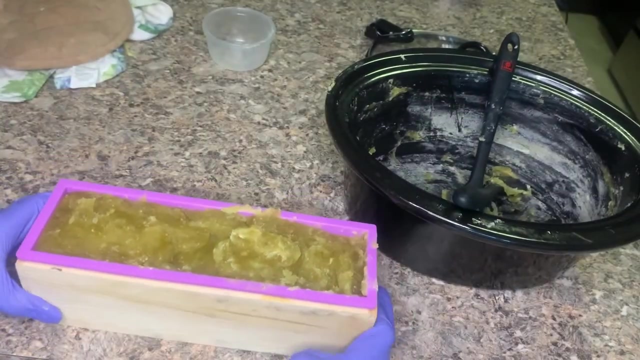 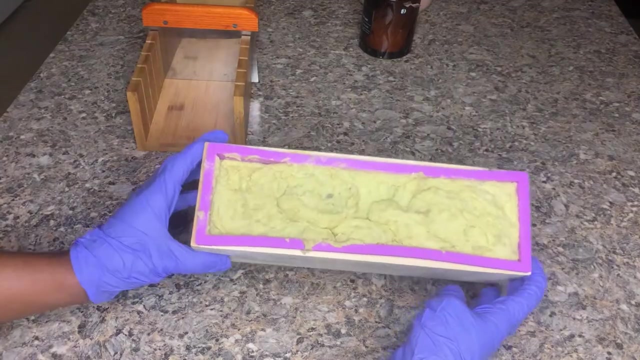 avoid any air pockets in your soaps. so I'm gonna mold and then I'm gonna shake, shake, shake, shake, mold, shake, shake, shake, shake, shake until I am finished. it's the next day and my soap is hard and it's ready to be cut. so the way that 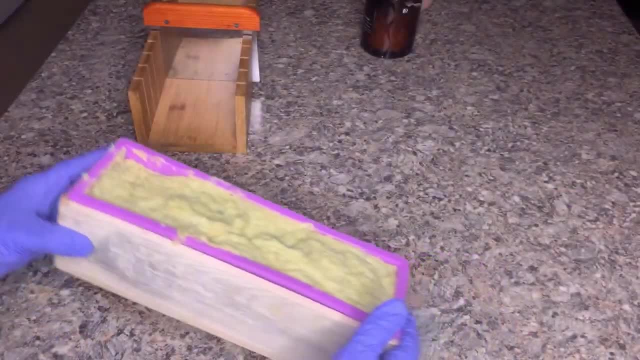 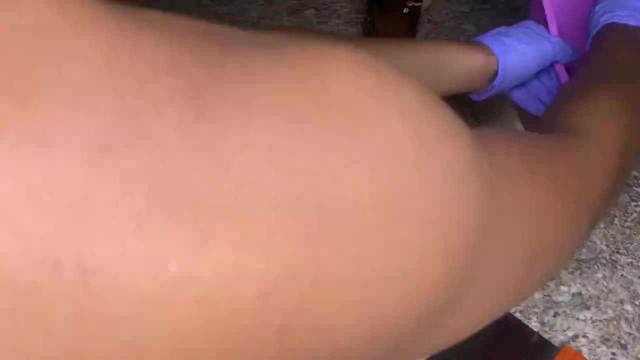 I cut this soap was. I used my soap cutter that cuts bars into four ounces, and I used a straight cutter and I just love this soap. I do let it cure for about one or two weeks but because of the hot process method the soap is ready to be. 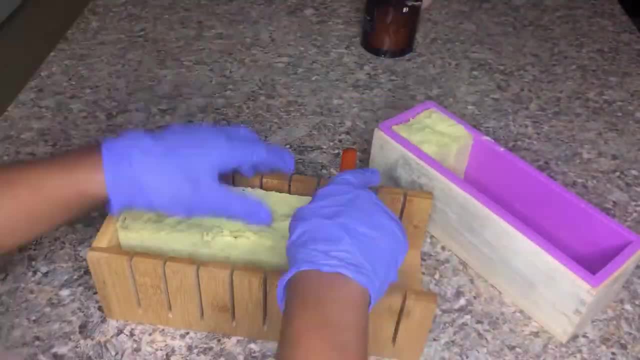 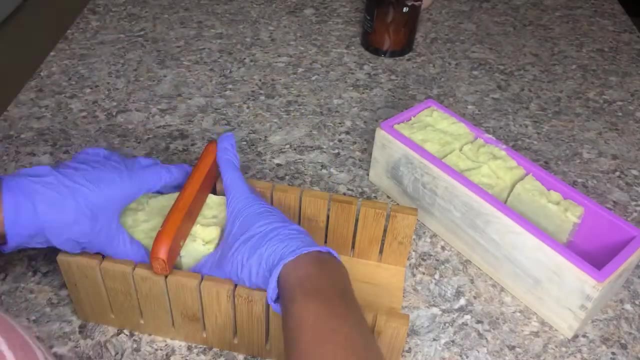 used as soon as it's cut. I just like to let it get harder and more firm by letting it cured for about a week or two. if you want to try any of these soaps, you can head over to my website. I do have some available and if you want to. 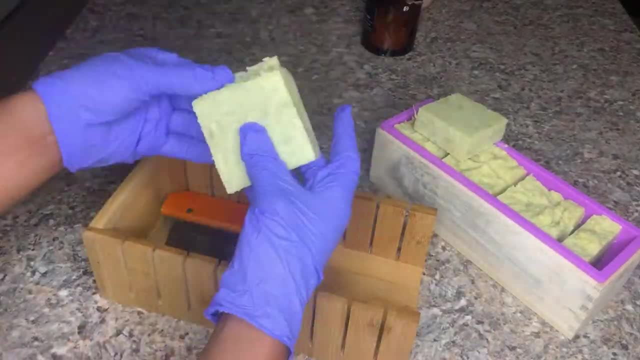 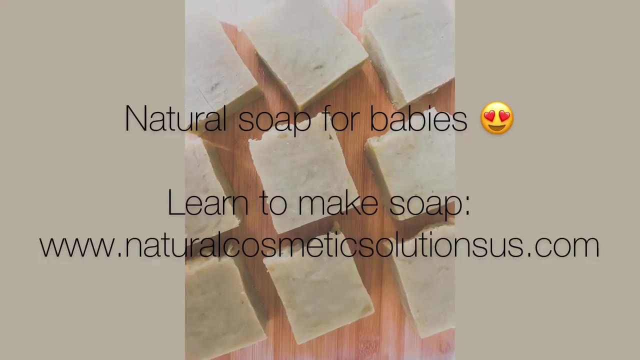 try and make this one head over to the site too, because I have the blog with the recipe listed. make sure you subscribe and I'll see you guys next time. bye you.